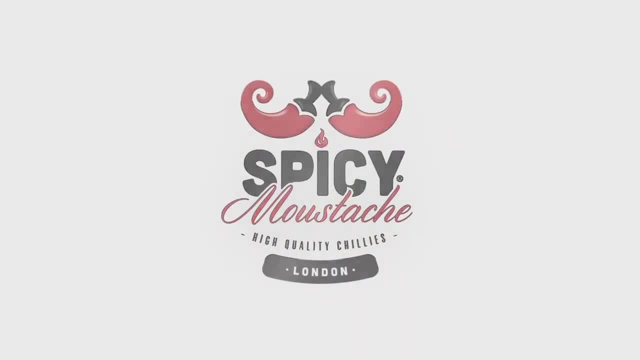 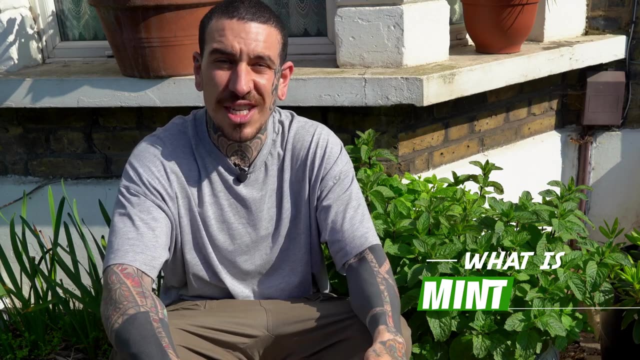 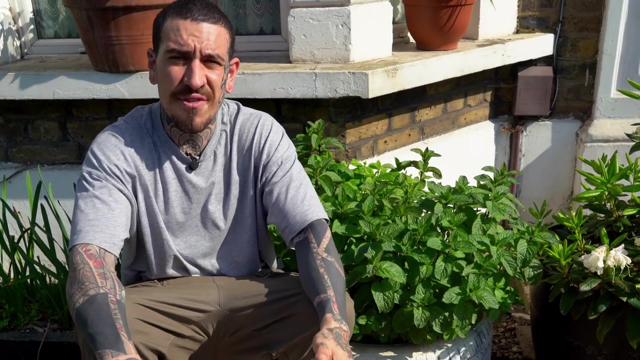 Mint is an aromatic herb that comes from the name mentha. There is a great story behind this brilliant plant Native to the eastern Mediterranean. mint gets its name from the nymphae mintae. Gelius Persephone turned her into a lowly mint plant after she had an affair with 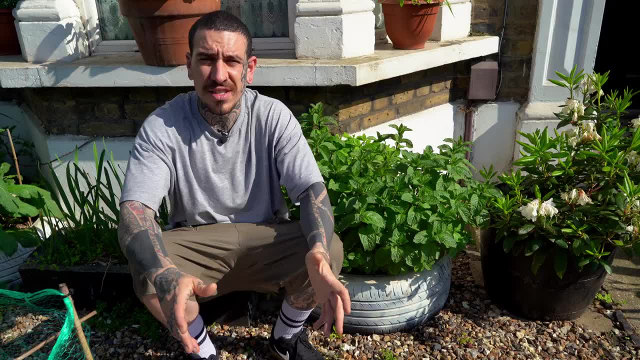 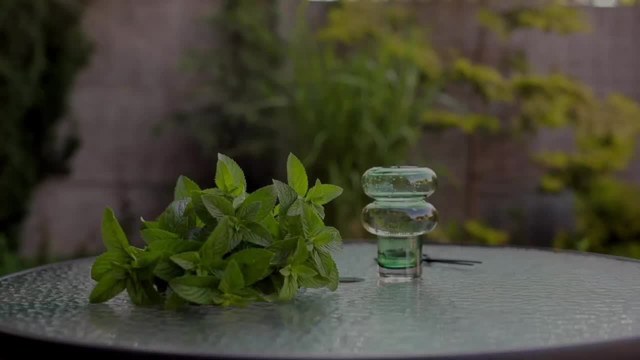 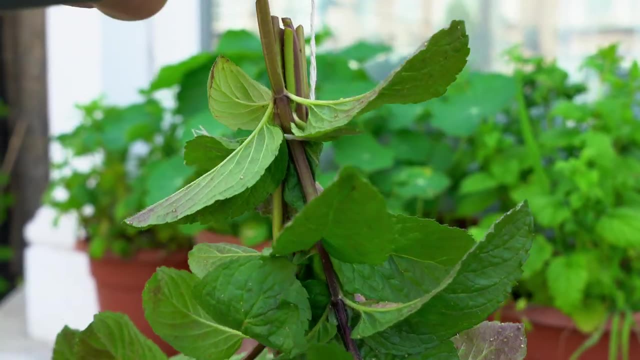 Pluto. The mint plant is common and the favorite of many gardeners, so it's easy to grow your own Mint taste is sweet and produced a lingering effect on the tongue. The fresh leaves have the most flavor and scent and I use them mostly to make tea or cocktails. You can store fresh mint in the refrigerator or you can hang. 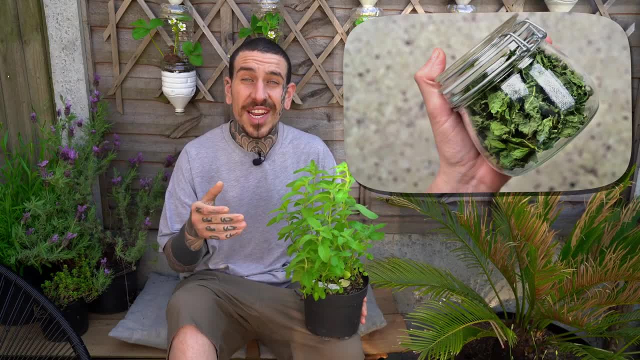 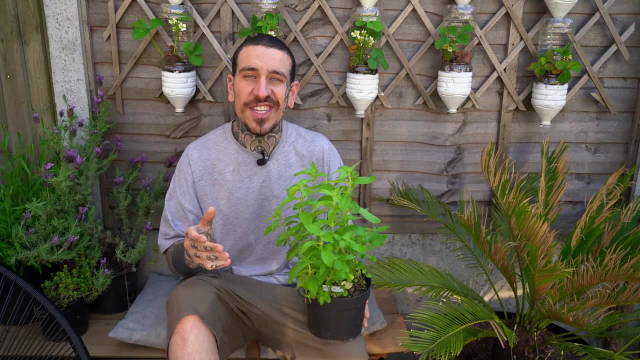 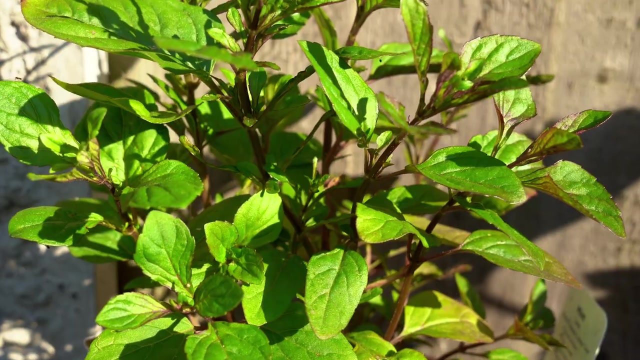 it upside down until dry. Once dry, store it in a jar or a sealed plastic bag. These allow you to enjoy mint all year round. There are many different strains of mint available and I'm currently growing a few, including banana mint, chocolate mint, ginger mint, lime mint, pepper mint. 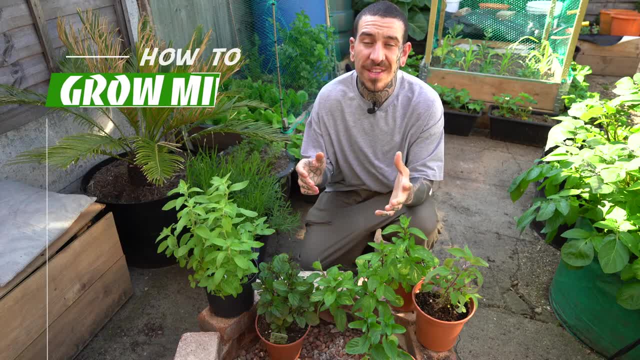 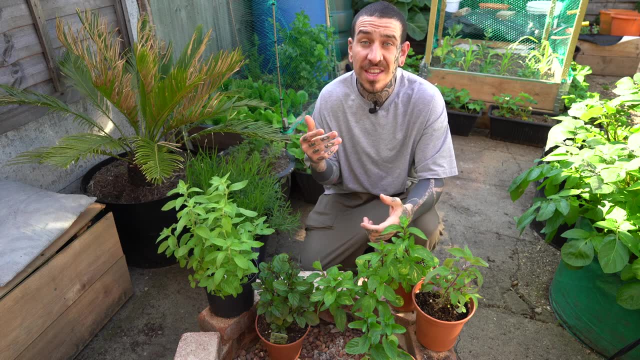 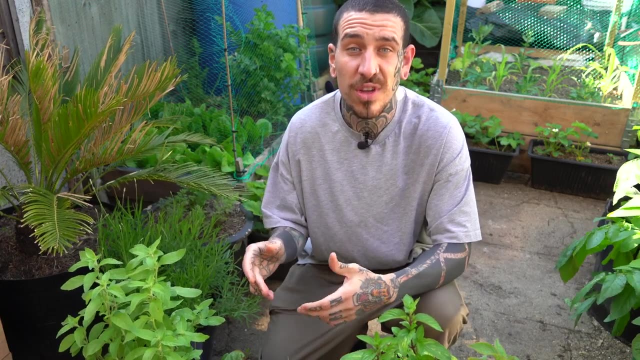 and my absolute favorite, pineapple mint. Avoid growing different varieties of mint close together, either in pots or ground, as they could potentially lose their individual flavor and scent. A few years ago, I made a mistake to plant mint straight in the ground in the only spot of open. 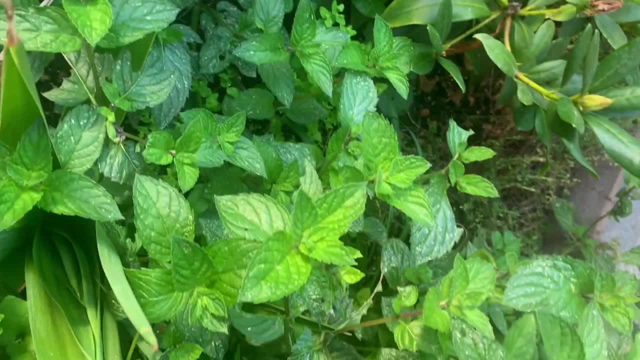 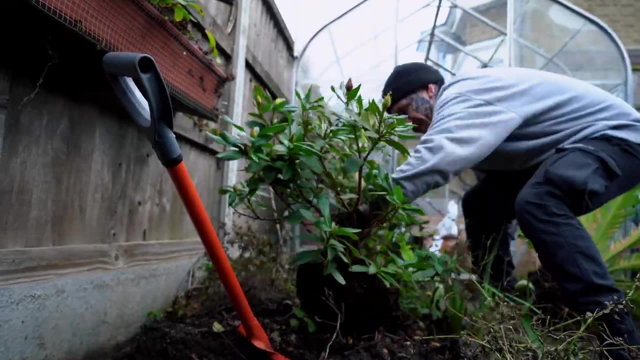 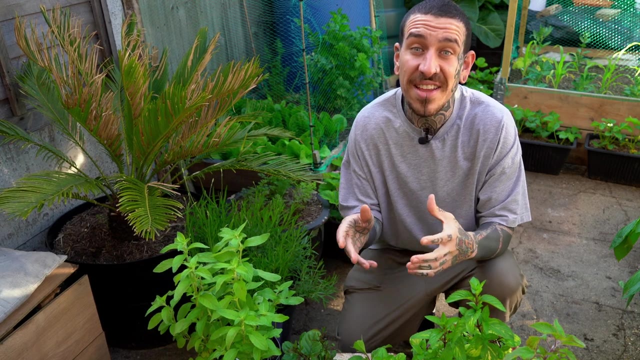 ground that I have in my garden. It took over the whole space and trying to control it was absolutely pointless. I had to remove all the existing plants and dig up roughly one meter deep sift through it. The reason is that mint roots spread easily because of the resilient rhizomes. 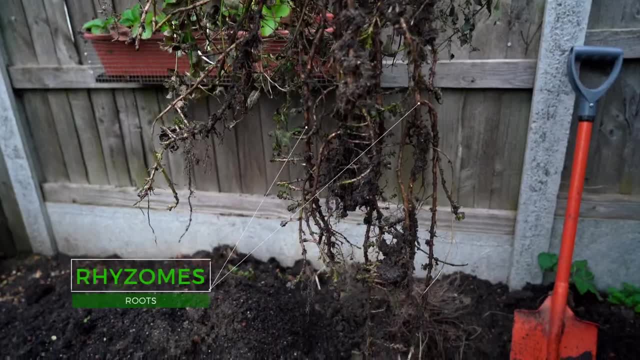 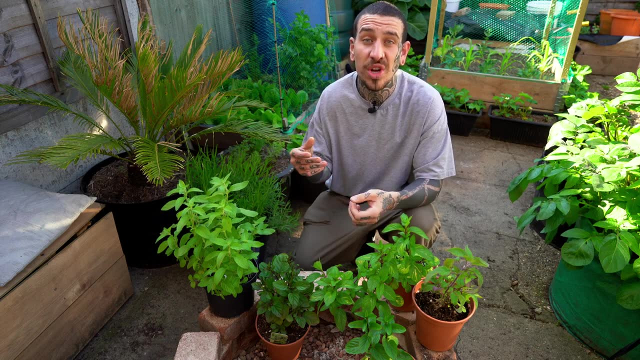 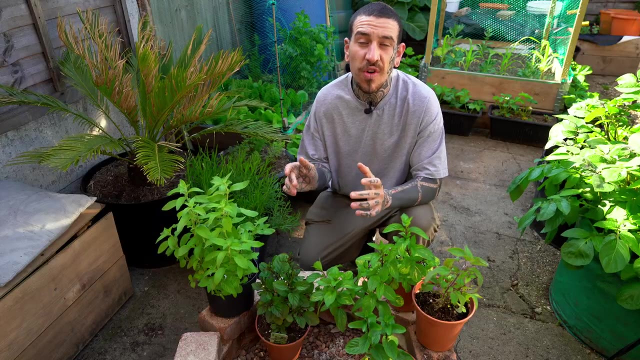 If you checked my video about ginger, a rhizome, it's a large underground stem that grows horizontally and shoots out roots and new shots. This means that even if a small bit of fruit is still in the ground, it will develop new shots. This is why you should always grow mint either. in isolation or in containers. It grows well in both full sun and partial sunlight. However, if you live in a hot climate, it's recommended to grow it in partial shade. Feed your mint with an organic fertilizer like well-rotted manure or a slow-release fertilizer. 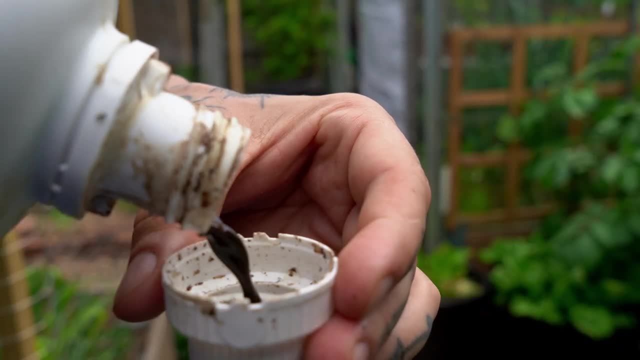 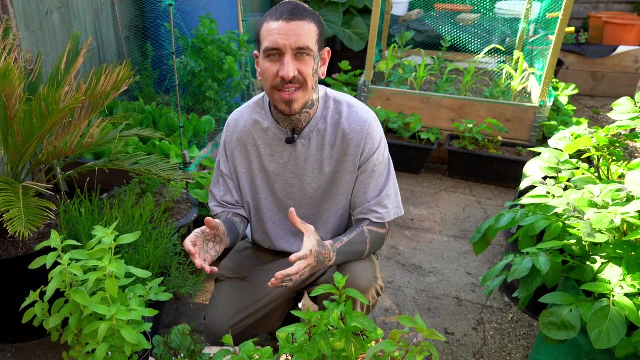 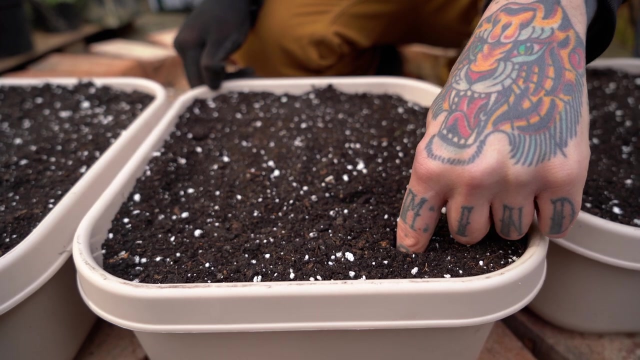 You should start feeding your mint when spring begins or roughly one month after you planted it. Water mint regularly and keep the soil moist but not soaked wet. A quick trick to understand if your plant needs water is to stick your finger into the soil and you can tell if the soil is wet or not. If your plant needs water, you can stick your finger into the soil and you can tell if the soil is wet or not. 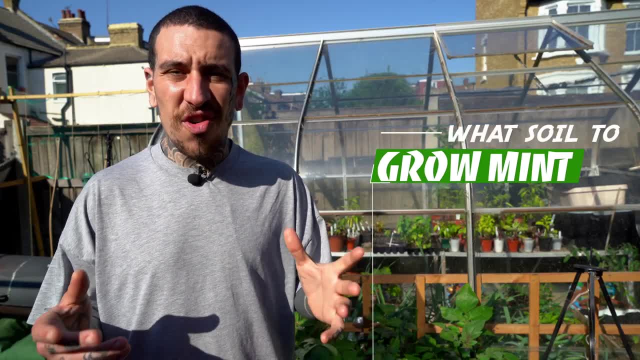 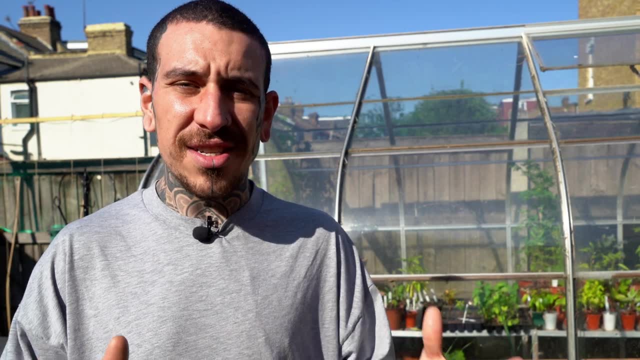 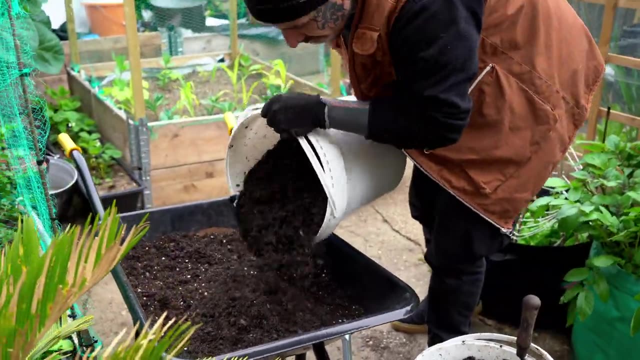 If it's dry or still moist. Mint thrives great in pretty much any kind of moist, well-draining and rich soil. I recommend to buy a pre-mix from your local garden center or you could potentially make your own. I make my own by mixing 50-50 good potting soil and 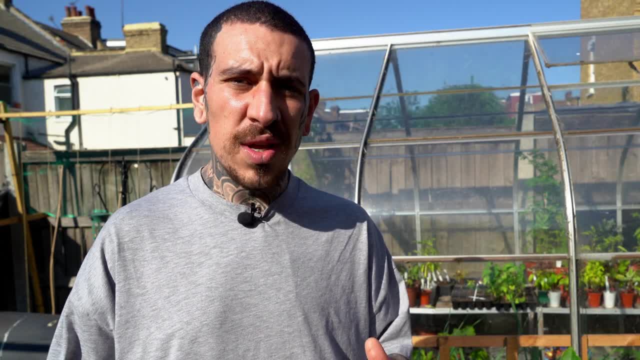 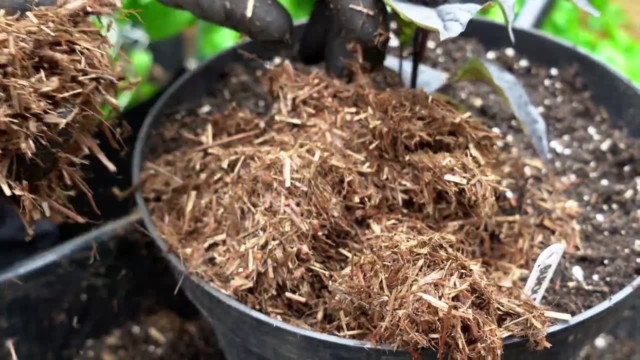 mature compost. You could also grow mint on your windowsill by using well-draining soil and slow-release fertilizer. I also mulch the soil to retain moisture and limit the amount of weeds that could potentially grow in the same area where the mint is growing. 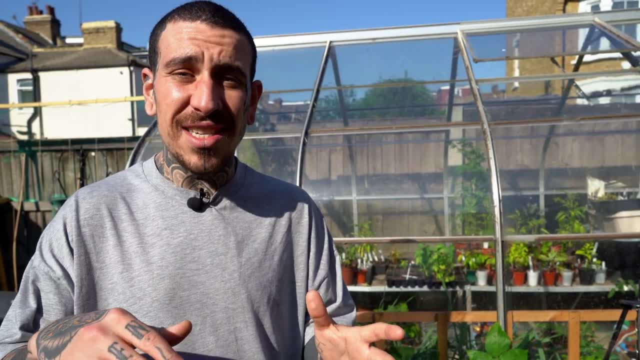 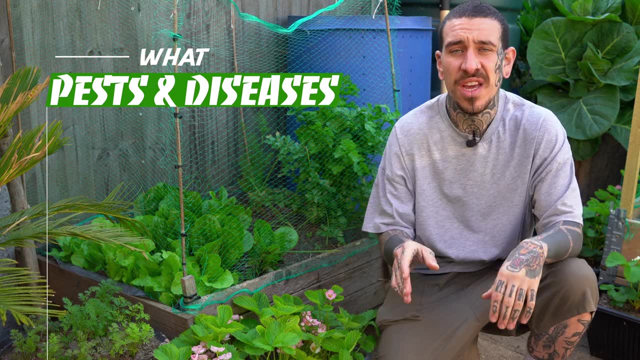 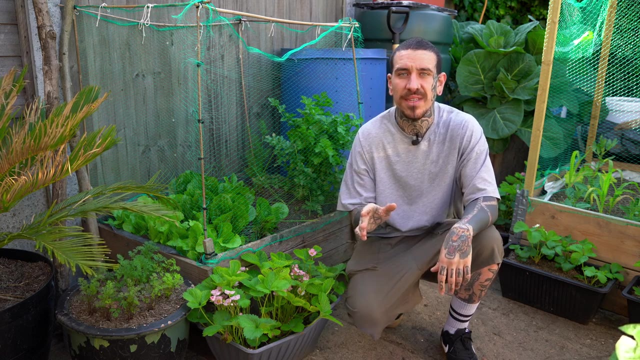 Spread around 2-3 inches of mulch around the base of each mint plant. Do not spray your mint with any kind of chemical pesticide. The residue of the pesticide could be easily ingested once you consume the leaves. However, there are many kinds of pests that could potentially attack your mint, For example. 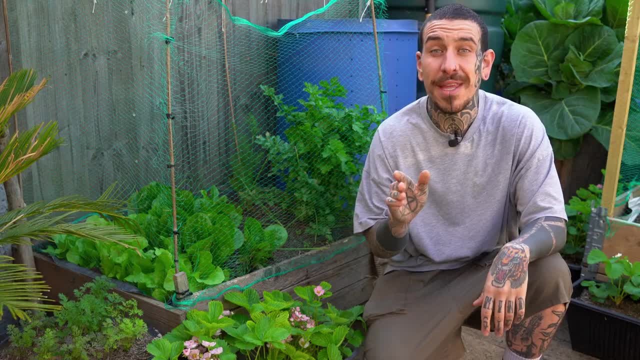 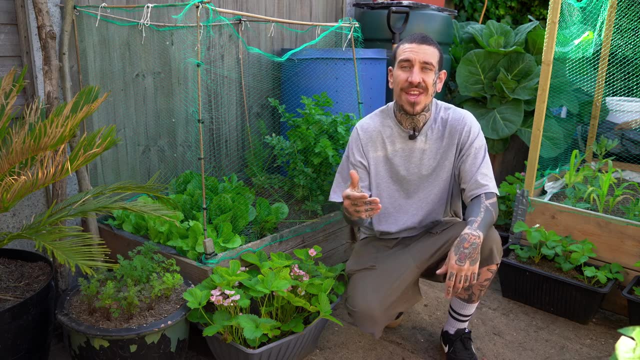 mites and aphids are a really common issue for mint plants. If you have a light infestation, you could potentially just spray your plants with a strong jet of water and this will get rid of the aphids. As a last resource, insecticide might be needed if there is a really strong infestation. Look for: 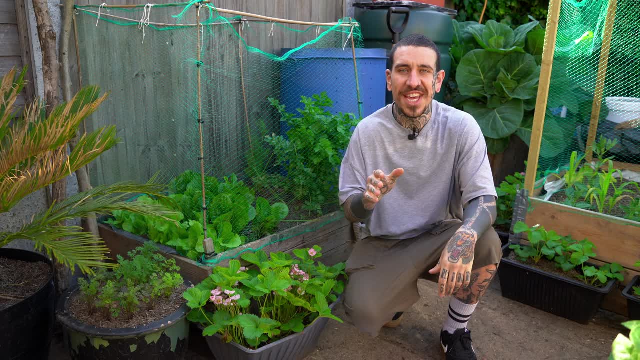 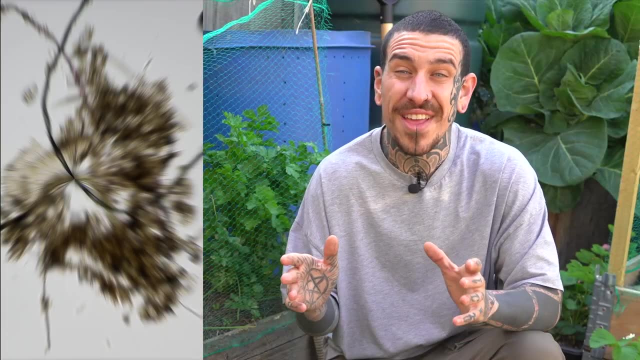 insecticides with imidacloprid. This will kill the aphids without harming any other beneficial insect, like bees and butterflies. I also use nematodes as a preventive measure. You could simply mix it with water and directly water the base of your plants or spray the leaves. 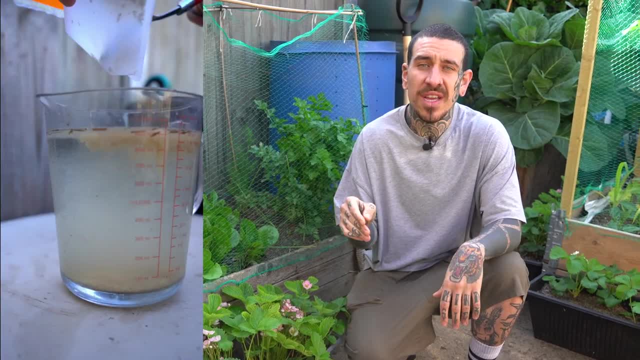 I personally noticed that two aphids were more effective than the other two. I personally noticed that two aphids were more effective than the other two. I personally noticed that two aphids were more effective than the other two If you have a large application of nematodes roughly at one month distance between each other. 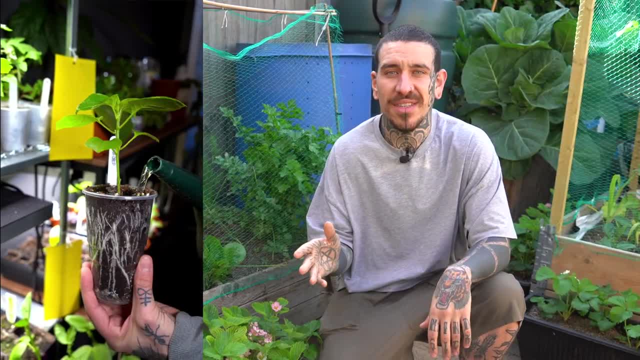 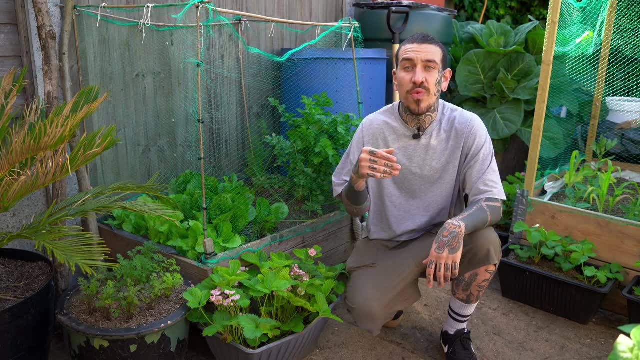 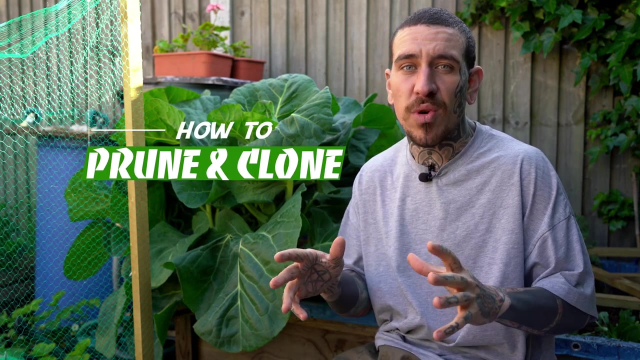 they drastically reduce the amount of pests attacking my plants. Natural predators like lacewings or ladybugs could be released at the beginning of the season, so you would have an organic pest control in your garden. Mint is a plant that grows really dense and sometimes much more than what we can. 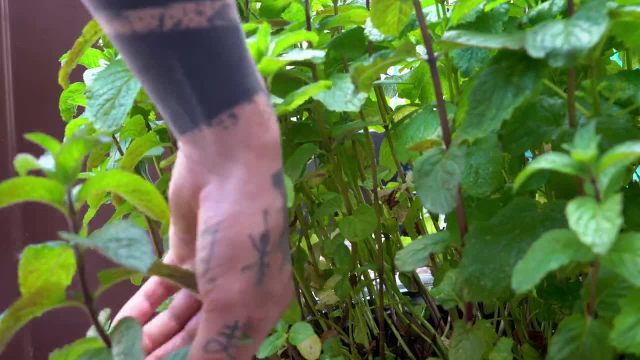 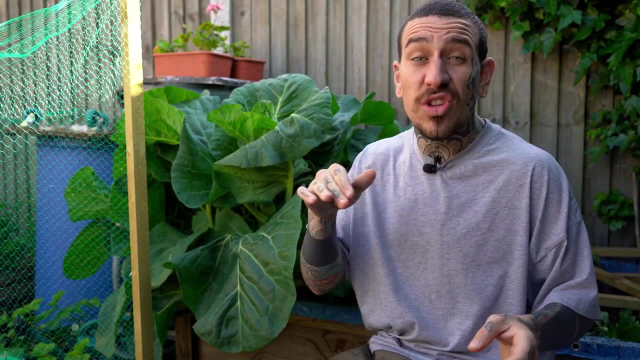 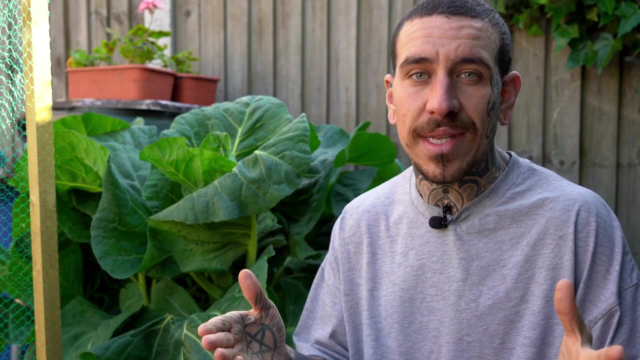 consume. However, even if you don't use it straight away, it's recommended to prune it down and store it for later use. You should always prune back lateral shoots and top up a few nodes. Your mint will benefit from pruning, especially at the end of the season when the plant is due to go dormant.